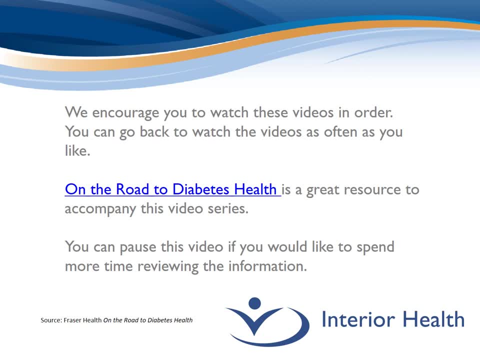 order and just remember you can go back and watch the videos as often as you'd like. Fraser Health On The Road To Diabetes Health is a great resource to accompany this video series. and remember you can pause the video at any time if you would like to spend a little bit more time reviewing the information We 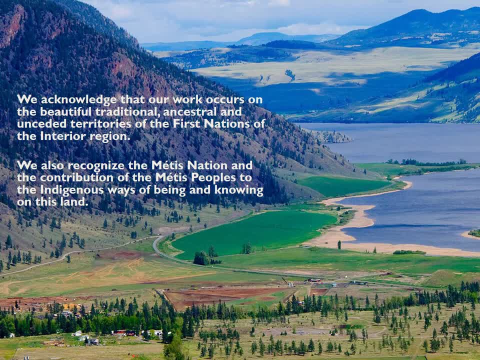 would like to acknowledge that our work occurs on the beautiful traditional, ancestral and unceded territories of the First Nations of the Interior Region. We also recognize the Métis Nation and the contributions of the Métis peoples to the Indigenous ways of being and knowing. 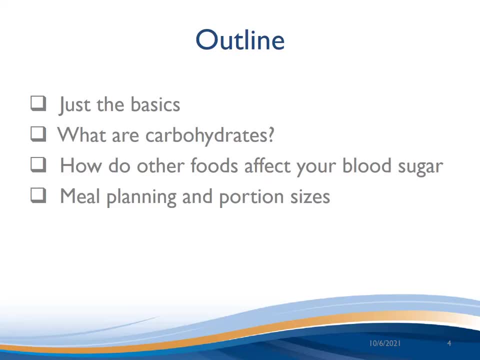 on this land. Today we're going to discuss the basics of nutrition and diabetes. what are carbohydrates? how do other foods affect your blood sugar and, finally, some ideas around meal planning and portion sizes. Let's get started. Remember that diabetes is a condition in 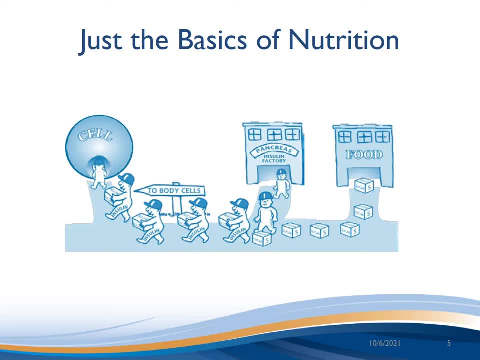 which your body cannot properly use and store food for energy. The fuel that your body needs is called glucose, which is a form of sugar. When you have diabetes, keeping your blood sugar levels within a target range is important. You'll need to work with your doctor to set up a blood sugar dashing and diet plan to get you. 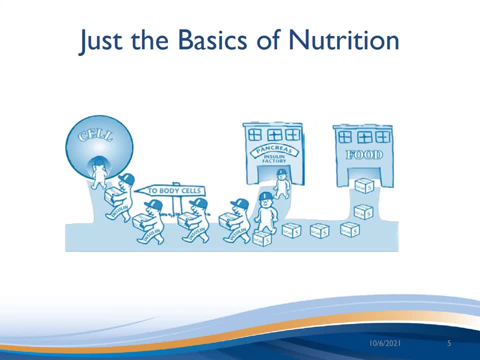 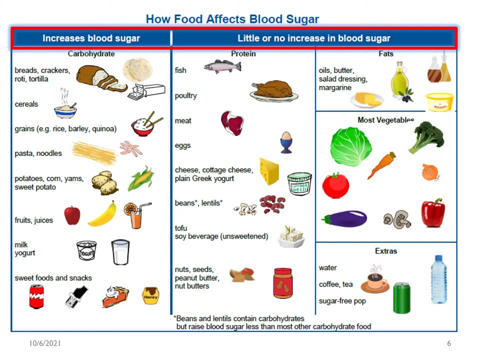 to set a blood sugar range. that's right for you. Now let's look at this chart about how food affects blood sugar. If you would like to spend longer looking at this chart, remember you can pause the video or view the chart in the On the. 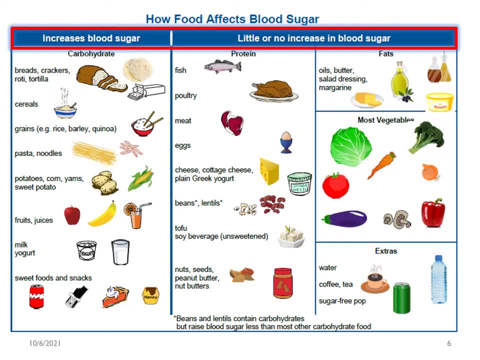 Road to Diabetes Health booklet, which is a resource we recommend to accompany this video. As you can see on this chart, the left side are foods that increase your blood sugars and on the right are foods that have little or no increase to your blood sugars. So let's look a little bit more closely at the sections. 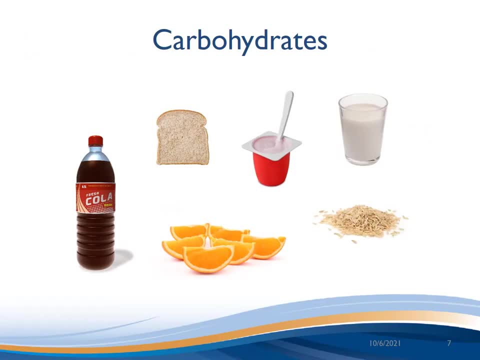 together. Carbohydrates, or carbs as many people call them, are what cause your blood sugar to rise the most. Tortillas, rice, potatoes, corn and beans are all examples of foods that are high in carbs. Other high carb foods. 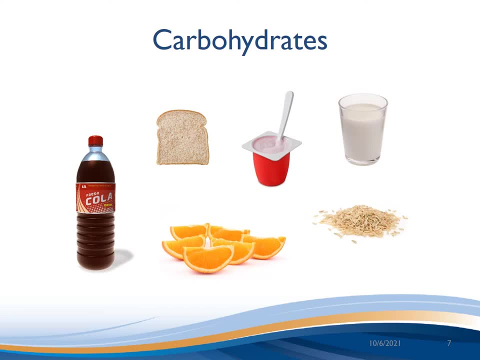 include fruits, milk and yogurt and sugar, sweetened foods and drinks. Even though carbs raise your blood sugar, that doesn't mean you can't eat them. It just means that you need to eat the right amounts at the right times In another 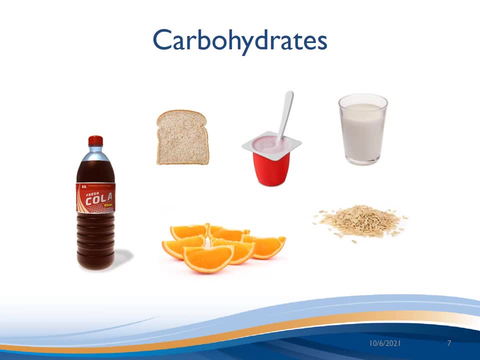 video, we will help you figure out how many carbs to eat each day. You'll also learn how to balance your carbs among your meals so that you don't eat too many at one time. Not only can this help you feel better, but it also helps prevent any future problems with your insader eyes. Easyup fits. 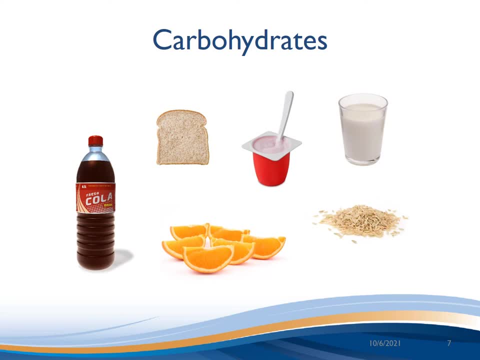 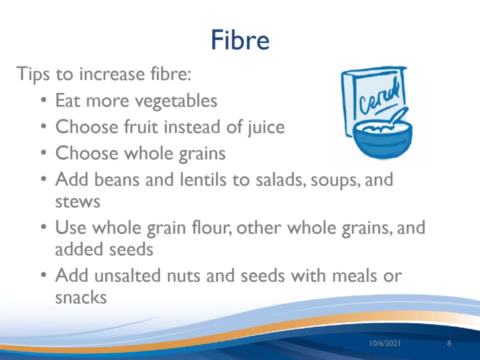 your body- nerves- I can walk- heart, kidneys and other parts of your body. Here are the 5 trends you can take into consideration when choosing carbs for your food. Food high in carbs may help you being full and lower your cholesterol week and blood sugar levels. Now it's important. 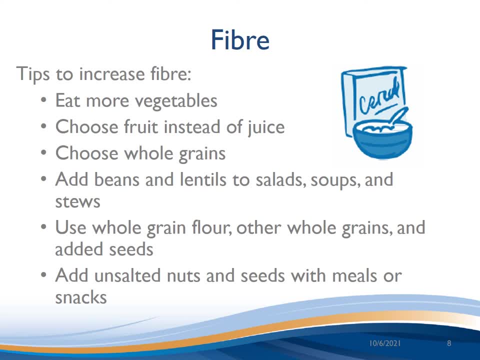 to choose. gains in carbs need Investment on carbohydrates that are high in level. fiber like whole grain breads and cereals, lentils, beans and peas is a good fruits. Vegetables are also an excellent source of fiber. A good amount of fiber to aim for. 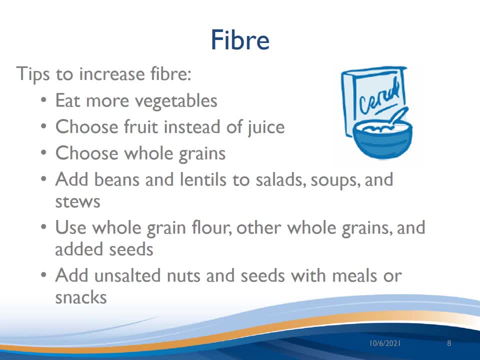 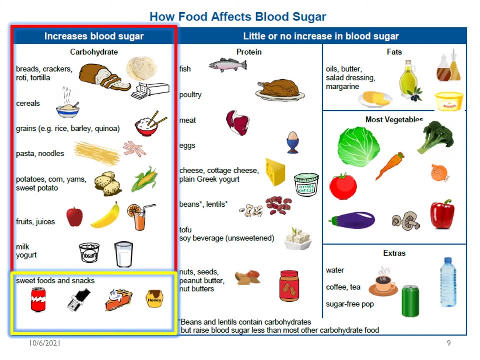 is 30 to 50 grams per day. It is important to remember that when choosing your carbohydrates, you should limit the amount of sugars and sweets, such as regular pop, desserts, candies, jam and honey, as the more sugar you eat, the higher your blood sugar will be Artificial sweeteners. 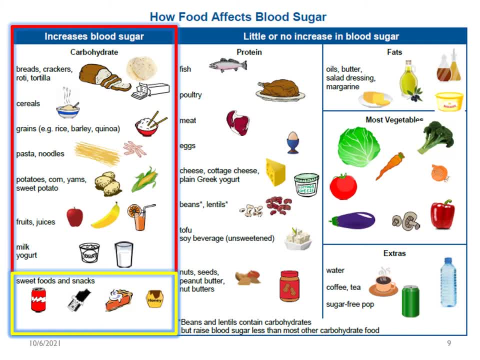 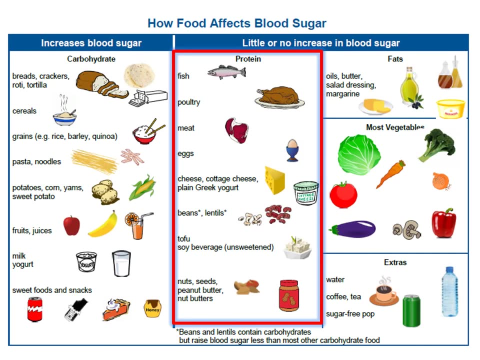 may be useful substitutes if you find it difficult to limit your sugar intake. Now that you know which foods contain carbohydrates and how they affect your blood sugar, let's talk about the other foods found on this chart. First, let's look at protein. Protein foods break down into only 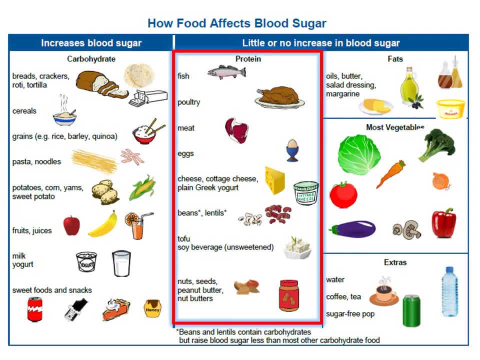 small amounts of glucose. When you include protein foods with your carbohydrates, it helps to slow down how fast the glucose is released. When you include protein foods with your carbohydrates, it helps to slow down how fast the glucose is absorbed. So we sometimes say that it helps to. 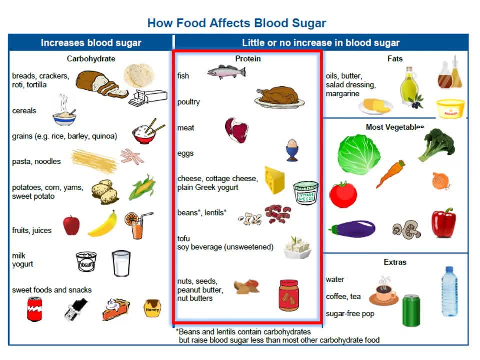 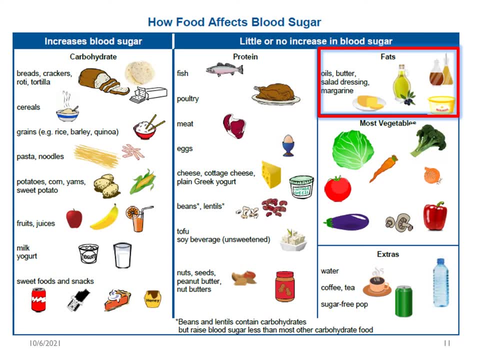 stabilize your blood sugars. Although some types of fat are important to include in our nutrition plan, you may also need to limit the amount of high-fat foods you eat, such as fried foods, chips and pastries, as high-fat foods may cause you to gain weight. A healthy weight helps with. 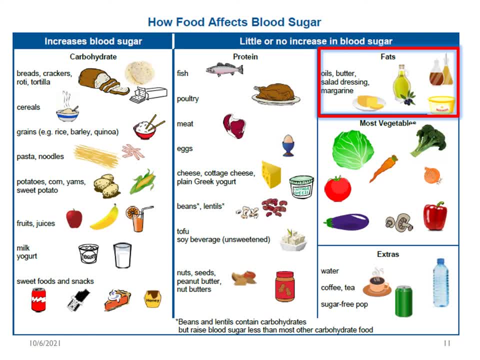 blood sugar control and is a good way to control your blood sugar. So if you have a high-fat food, it's healthier for your heart. Now let's talk a bit about vegetables. The good news is that most vegetables won't increase your blood sugars, so you can eat as much as you want. The only 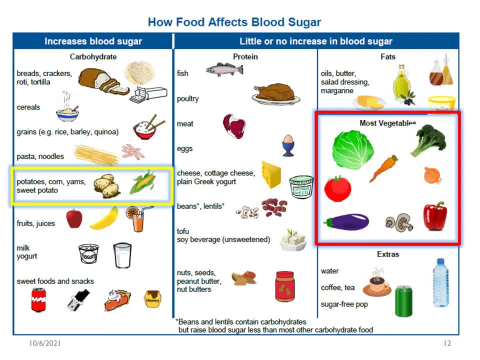 exceptions are the starchy vegetables like potatoes, corn, yams and sweet potatoes. Those are now considered carbohydrate foods and you will want to watch the portions of these: Lettuce, cucumber, onions, mushrooms, broccoli, cauliflower, bell peppers and zucchini. These vegetables will not. 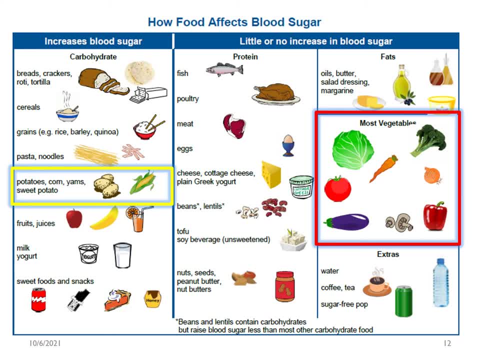 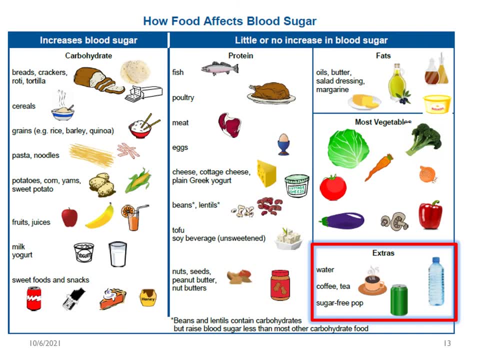 only help keep you full. they offer many important vitamins and minerals to your diet, as well as fiber. The last section on this page are the extras. Water, plain coffee or tea and diet pop will not cause your blood sugars to increase. Now that we have discussed foods and how they 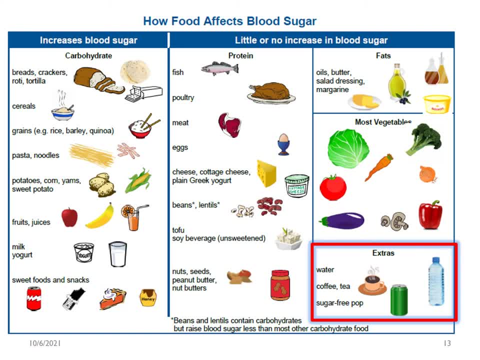 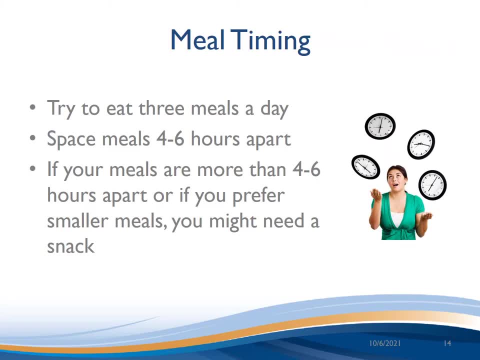 affect your blood sugars. let's move on to discuss other basic tips for healthy eating and diabetes. Meal timing can play a big role for healthy eating and diabetes. Try to aim for eating three meals a day and spacing meals no more than six hours apart. This is because eating 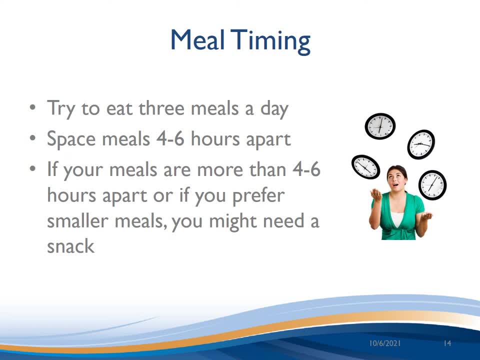 at regular times helps your body control blood sugar levels. We will talk about snacks later, but keep in mind that not everyone needs to eat snacks, but for some people they can help with keeping your blood sugar stable if you tend to space your meals far apart. 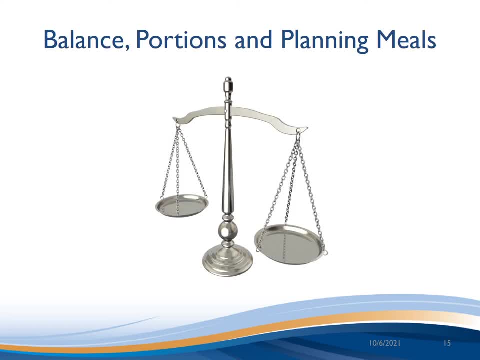 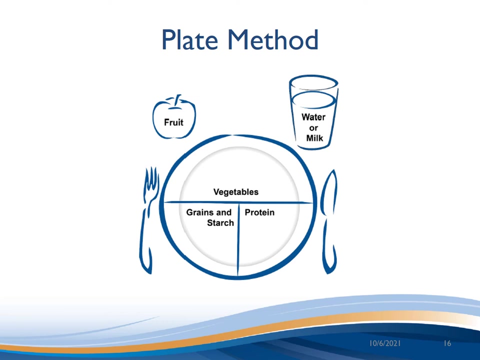 Now that we know how specific foods affect our blood sugars, let's review a few strategies to understand portion sizes and what a balanced meal looks like When you have diabetes. using the plate method can make healthy eating something you do and not something to count. the plate method helps you find the right balance. 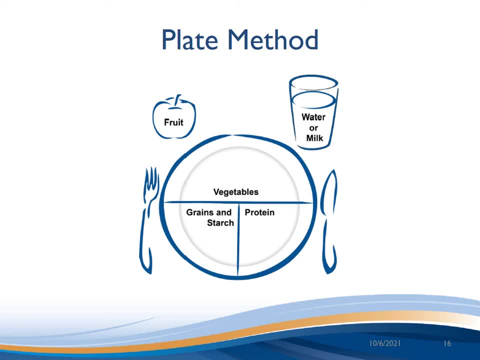 of carbohydrate, protein and fat. that can help you keep your blood sugar at a target level. the plate method is a way to build your plate with food. it uses healthy portion sizes of foods. you like to create a meal that's balanced for your health. your plate should be about 9 inches or 22 centimeters across. 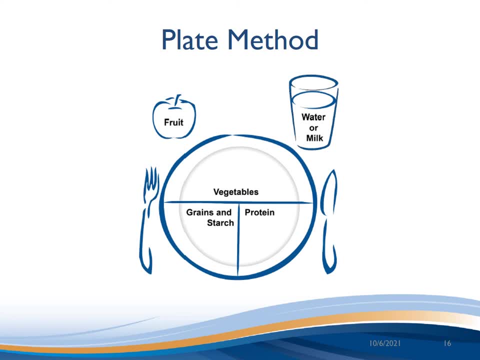 this may seem smaller than you're used to, but you get to fill it up. now let's check what's on the plate. a healthy plate has balance. about 50 percent is non-starchy vegetables, 25 percent is protein and 25 percent are starchy vegetables. 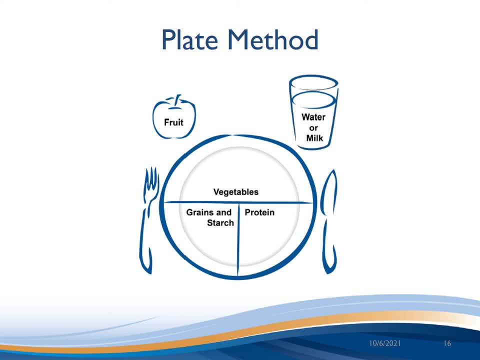 or breads, grains, or even fruit or yogurt. here's what that means. put the non-starchy vegetables, such as a green leafy salad or broccoli, on half the plate. The protein, like eggs, chicken, fish or tofu, goes on one-fourth of the plate. In the other fourth put a grain like brown rice or a. 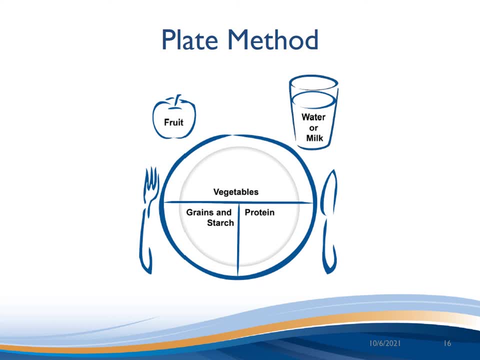 starchy vegetable like corn or some sweet potato. Hmm, maybe you're wondering if you will still be hungry. For some people, you may be able to add more carbohydrates to this meal, but try to choose a variety of carbohydrates. For example, if you eat rice with your meal, then you can add a piece of fruit or 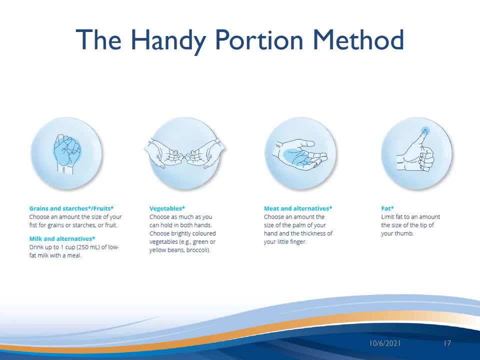 milk or dairy alternative. Another tool you can use to measure portions are your hands. The size of your hands can help determine the right portion for you. so make a fist and have a look. This is the right portion for you when choosing your carbohydrates, whether it is rice, pasta or fruit. Next, look at the size of 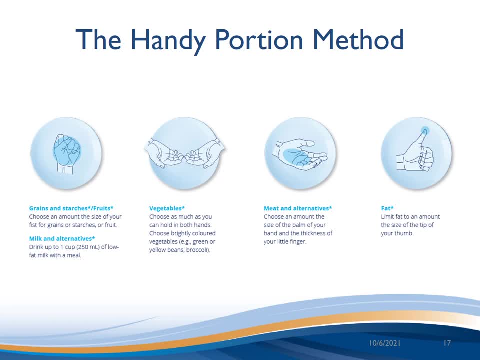 your hands so that you can measure the correct amount of carbs. If you have a of your palm, Without considering your thumb or your fingers, this is a good serving of protein food like meat, chicken or fish. Consider the thickness of your protein to.